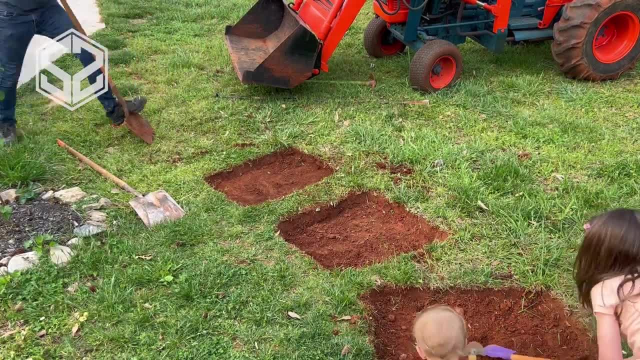 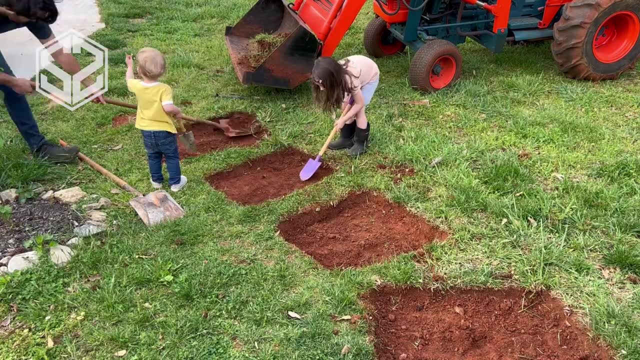 more jagged and sharp, and then the size changing from each paver, and they're going to be unique and different for each one. Now you may be thinking it might just be easier to purchase these large stones yourself and just lay them down without having to do all the concrete, which. 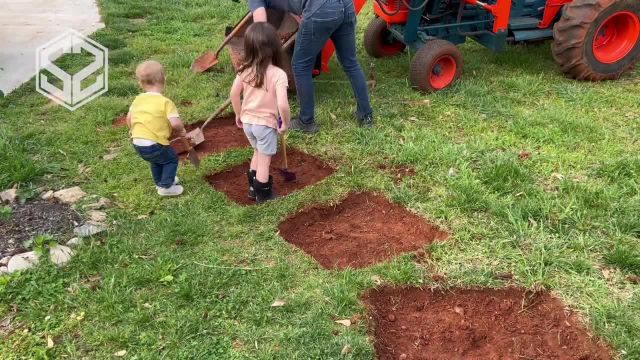 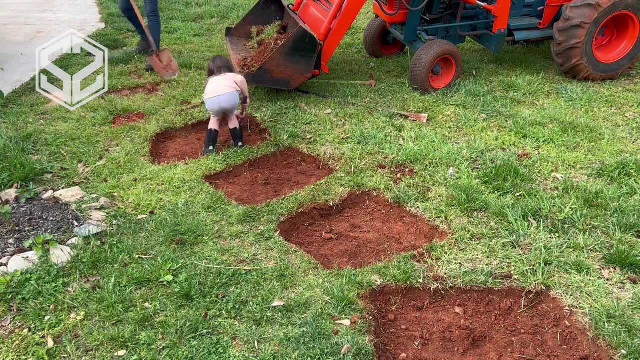 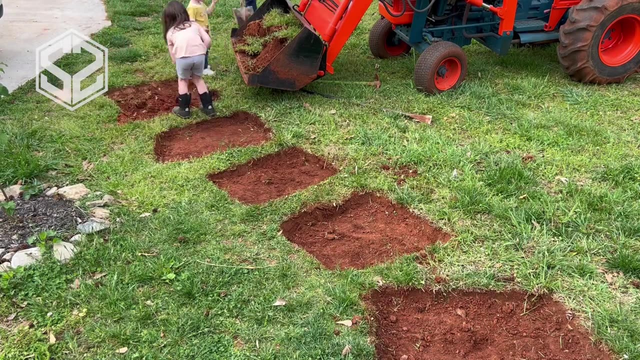 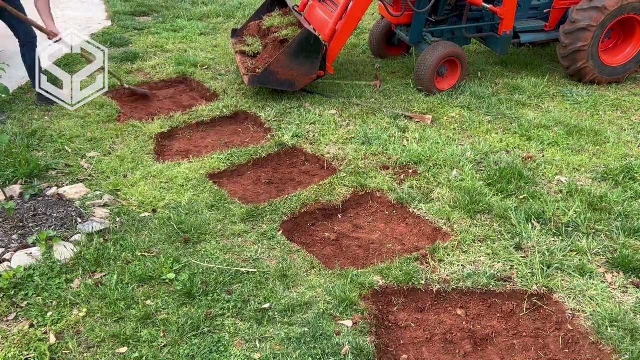 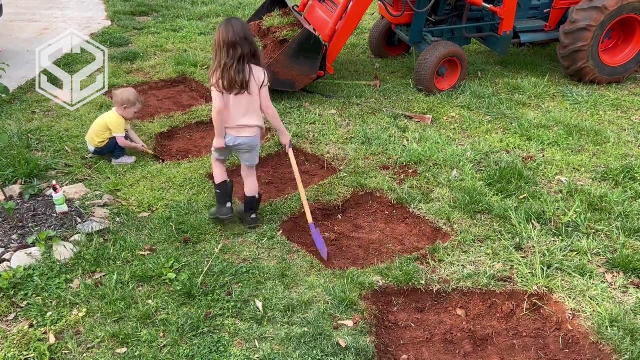 that's true, but where I'm located, it's really hard to find large slates like this. So I've just got a tool called the board. So what I'm doing here is I'm going to dig a little bit deeper to see if there's any. 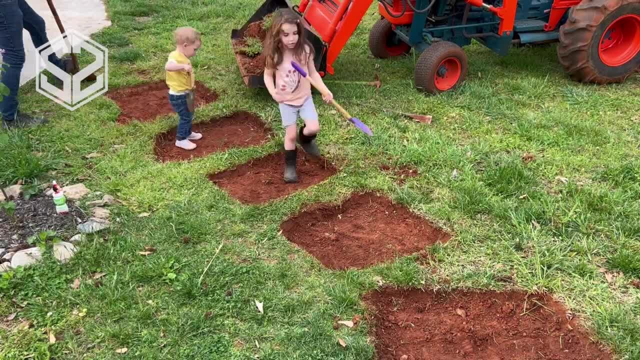 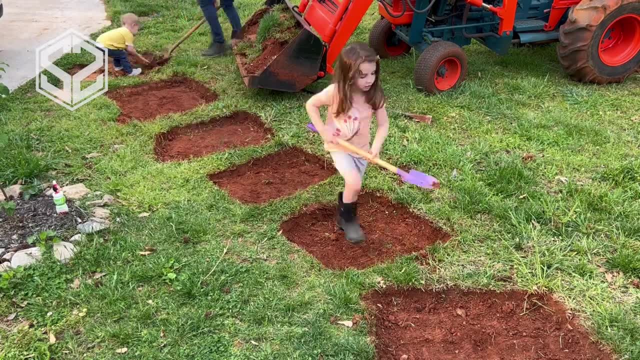 wood on the surface. So I've got to find a piece of wood that's more like a beam of light and I'm just going to cut down on part of the wood and I'm just going to cut down on it and I'm just going. 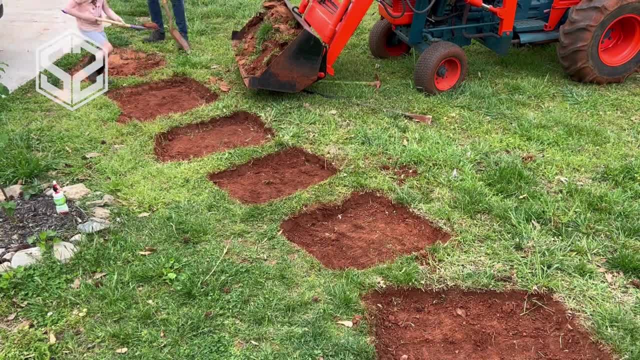 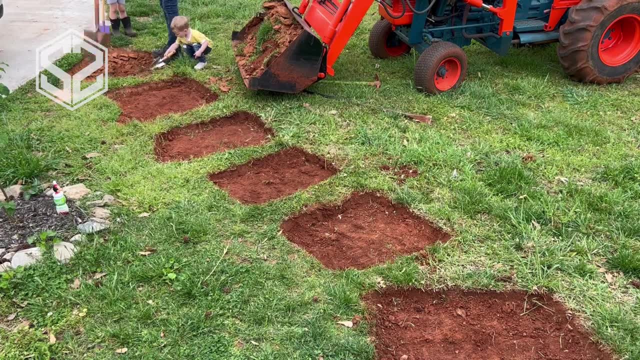 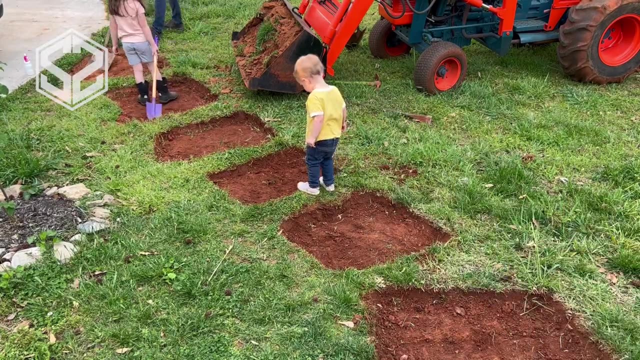 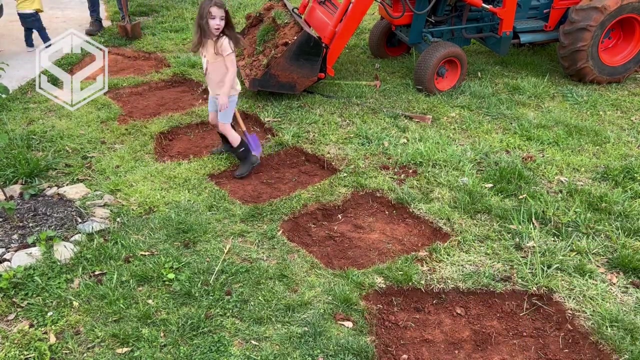 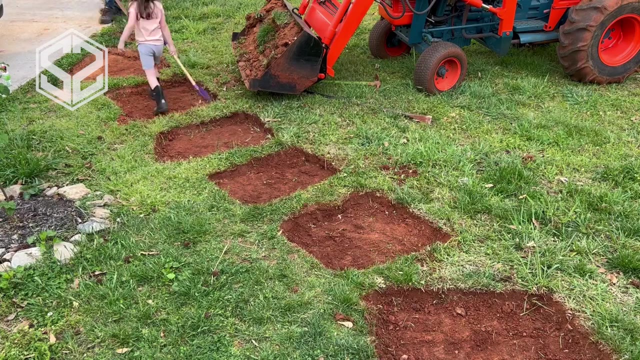 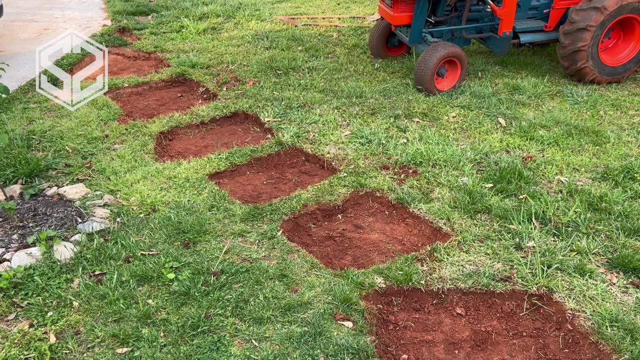 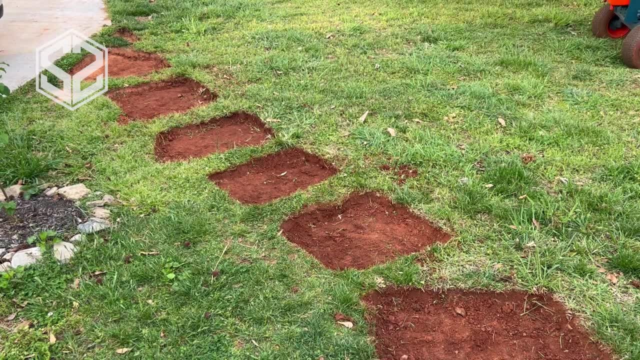 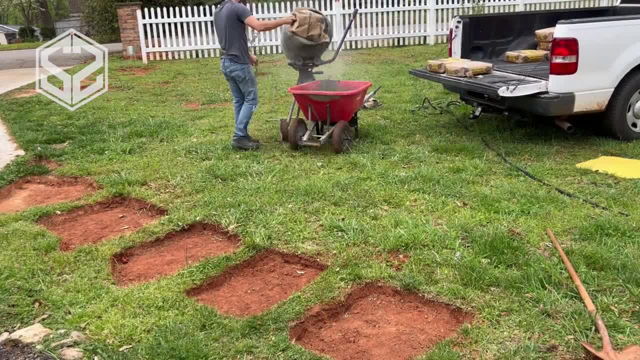 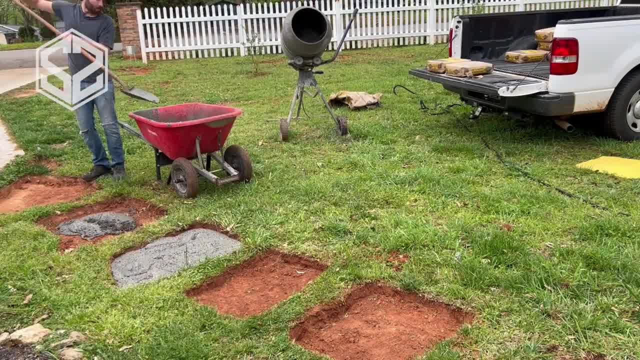 to cut this off. See Thank you. Next, I'm also going to be paying attention to the height. as I'm pouring the concrete, I want this to be pretty much level with the height of the grass, not the soil level, but a little bit above the height of where I'm going to be mowing the grass, because I want the stone to stand out from the grass. 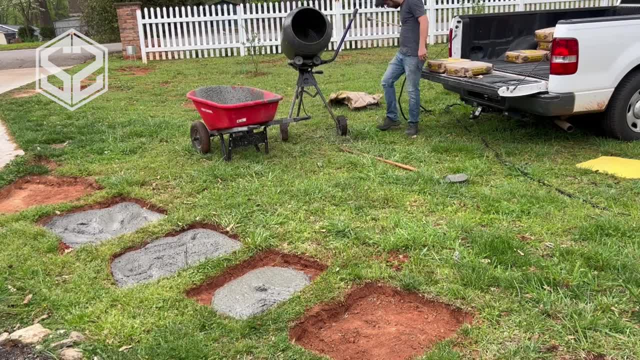 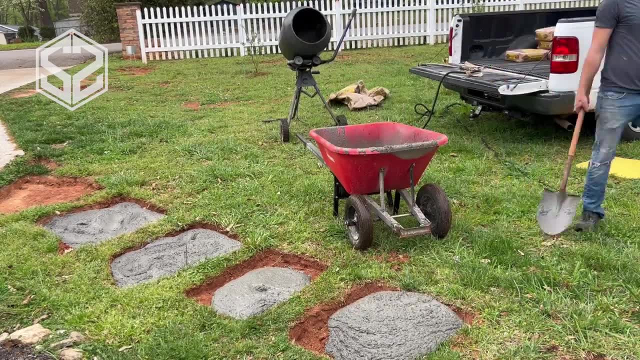 I don't want it to, over time, just get buried by the soil around it and just be a pain in the butt to have to edge around each of these stones. so I'm going to have it stand up out of the soil about an inch or so. 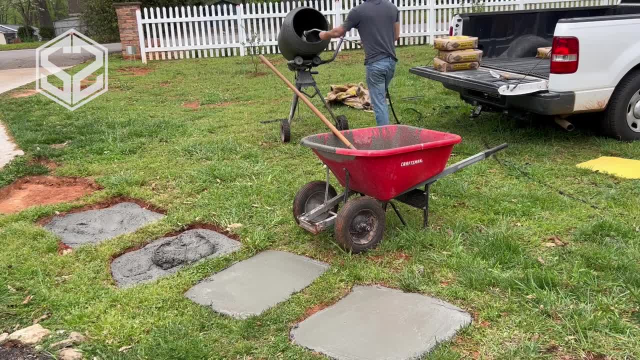 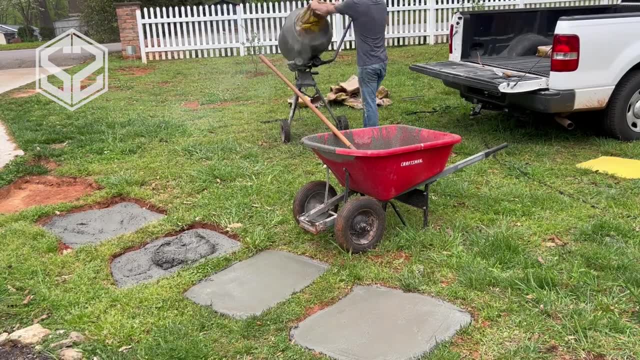 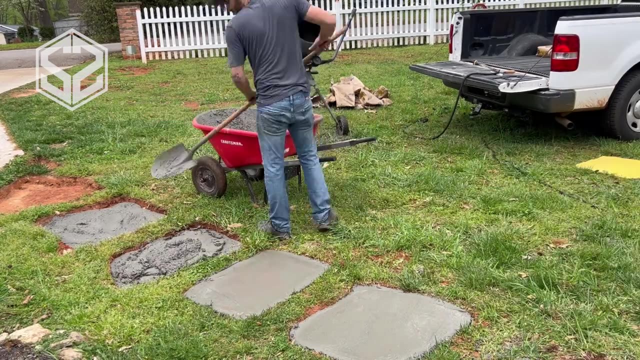 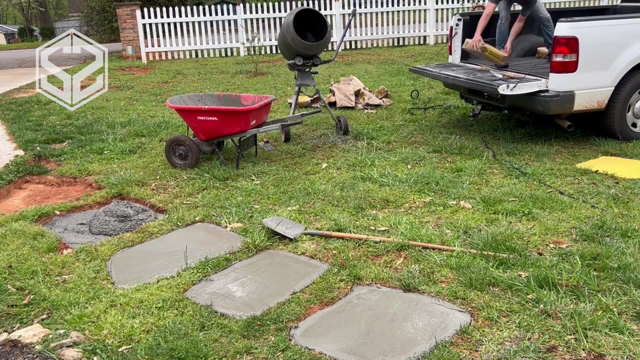 It's going to be a bit on the side, with the음덟Г Rhodes on the right. let's plant the Ivy así. Yes, I've already got a couple here and found this, but I've already gotten four with a 16, except when I was weighing it at the point when I didn't want to start planting them. 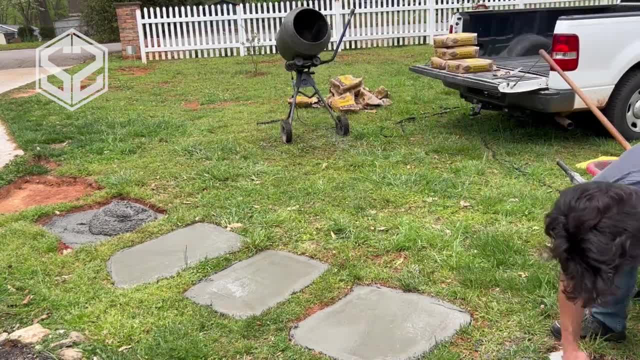 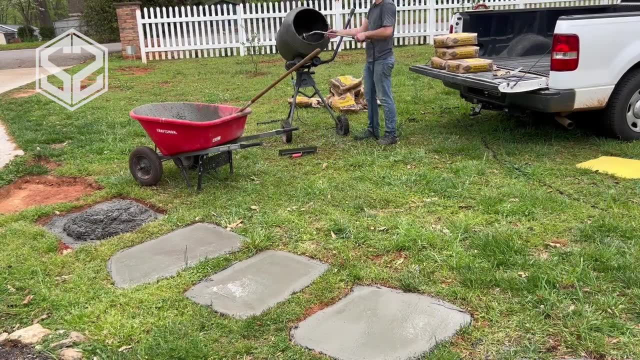 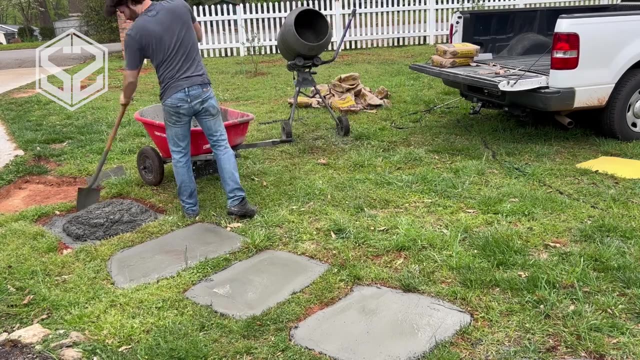 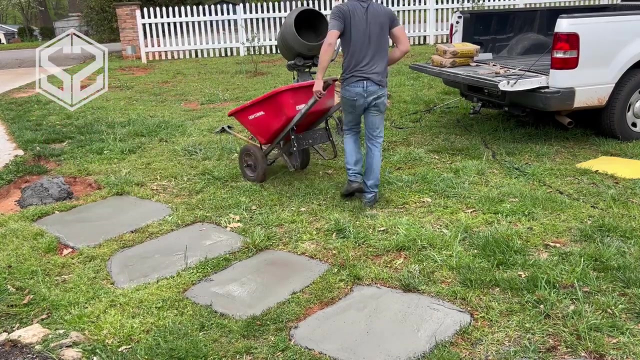 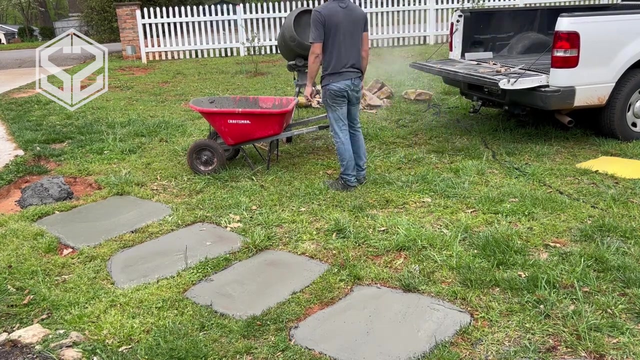 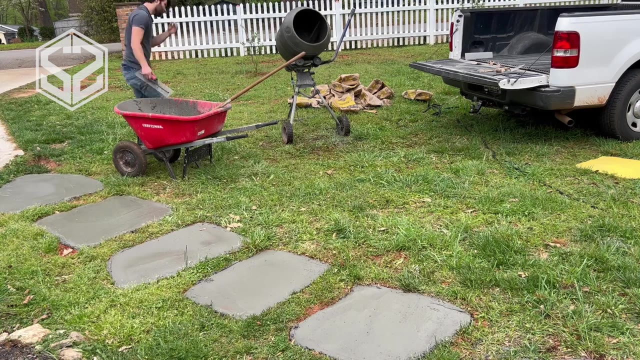 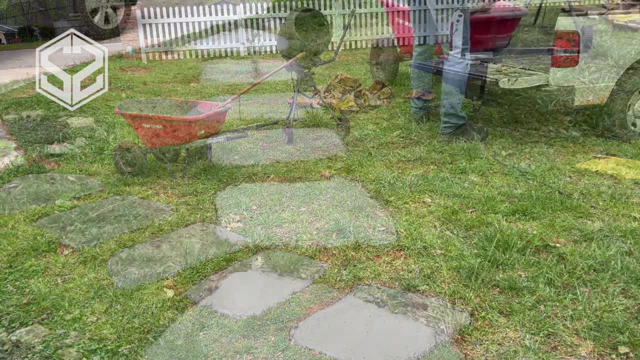 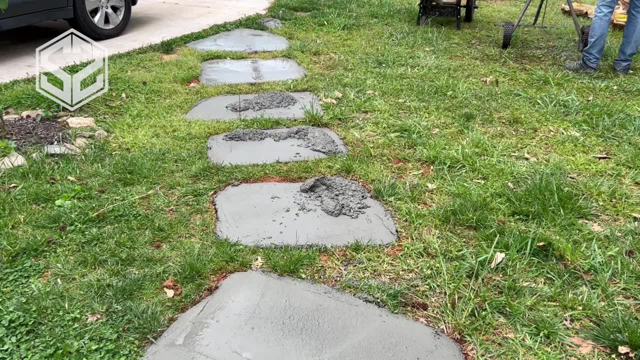 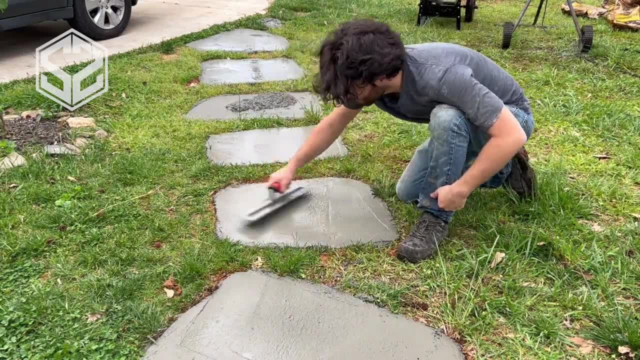 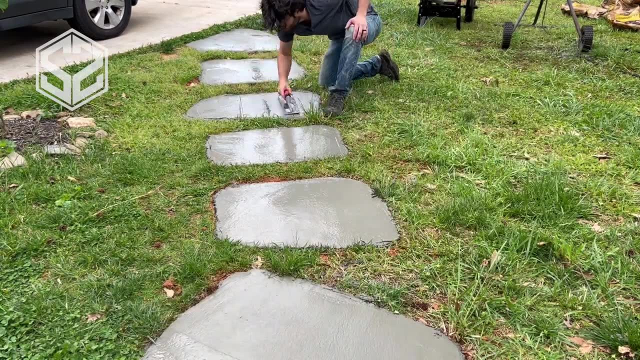 I need a little bit more concrete And a few of these sides. So I'll smooth those out again with the trowel And then I'm going to come back with some mortar in just a minute And I'll sprinkle that on top just very lightly. 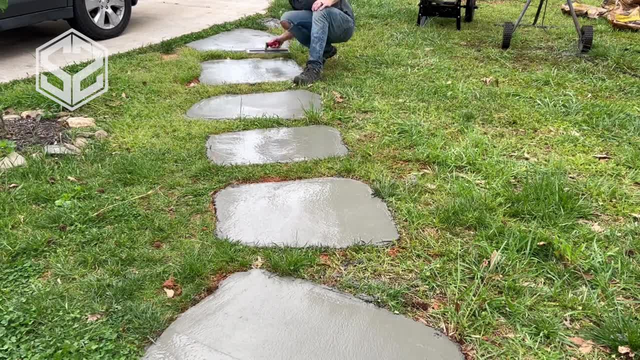 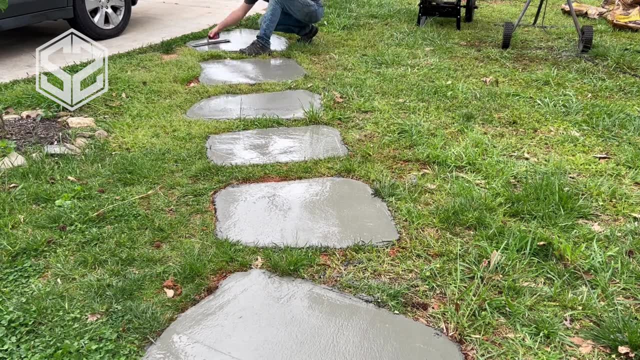 And basically mortar is concrete. It just doesn't have all of that large stones or gravel inside of it, So you can have a lot more control while you're trying to smooth over that surface. So this will help just absorb some of the excess water that's on top of the concrete. 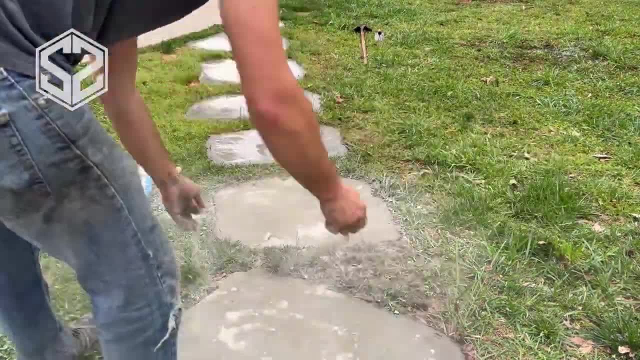 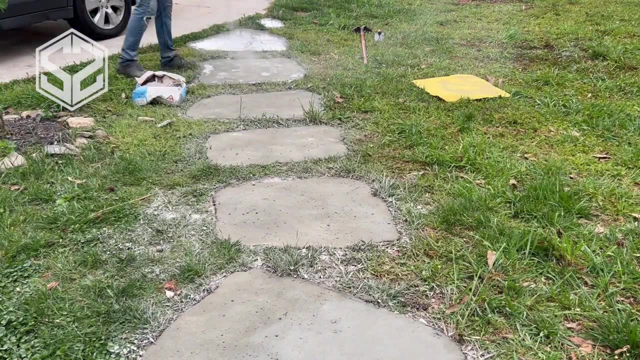 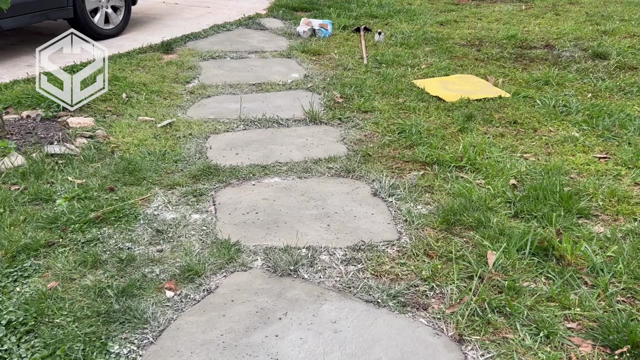 But it will also give me a little bit more freedom to sculpt and move things around Without the stones getting in the way as this hardens up. Next I'm going to come back with a small trowel And I'm trying to square up all of those edges. 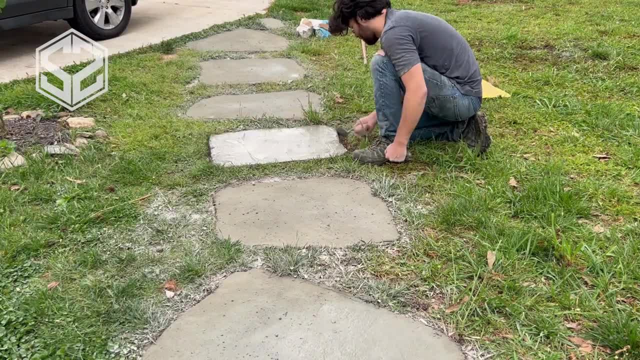 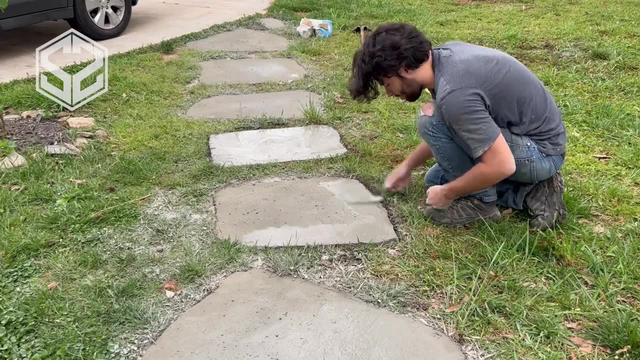 And this is when I'm really shaping the stone, Making it look more like a stone instead of a blob of concrete. So I'm going to go around all those edges and straighten those out, And then I'm going to add in some texture. 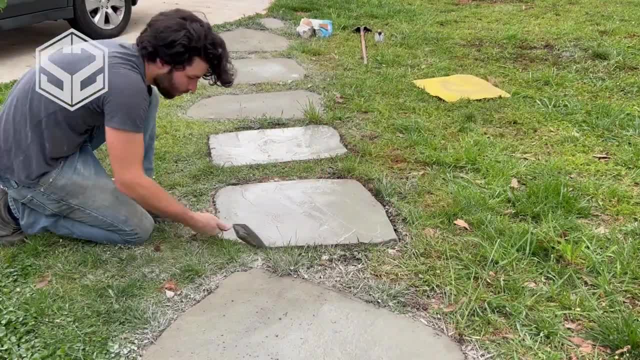 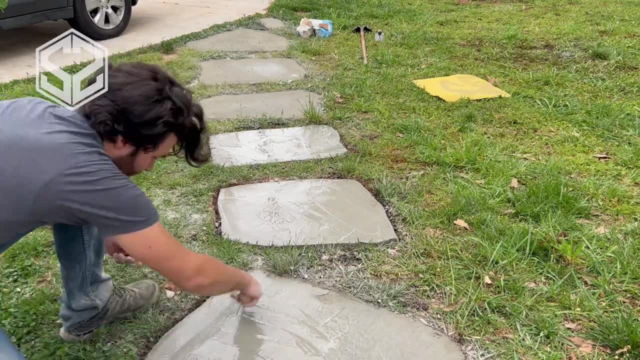 Some corners that are changed, Chipped off Different things to make it look more like a stone, And I think this is the fun part, Because not every stone has to be exactly the same. It doesn't have to be perfect, You can just have fun with it. 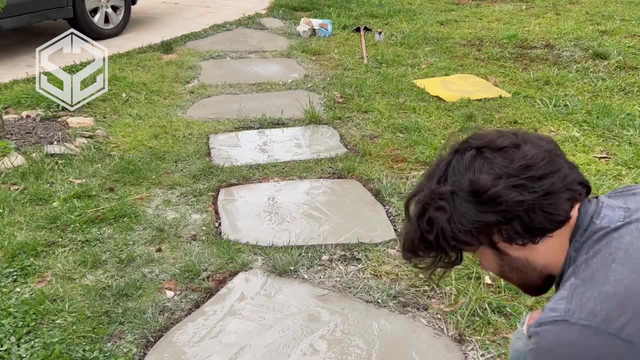 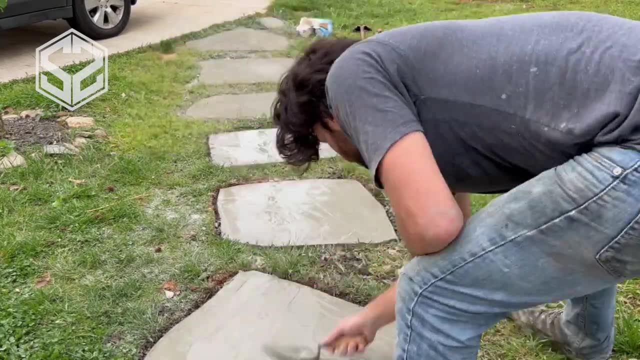 And you can see, while I'm doing this, I'm also smoothing out the top of the stone with that small trowel, And this time it's a lot smaller trowel. I'm leaving purposeful texture in there, Not making it perfectly smooth. 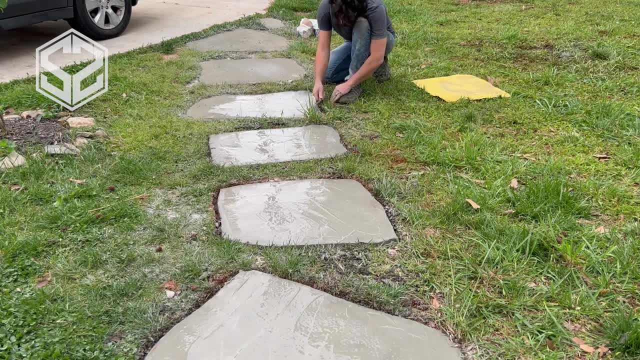 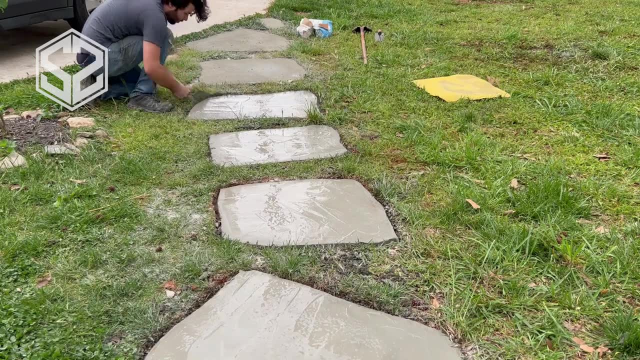 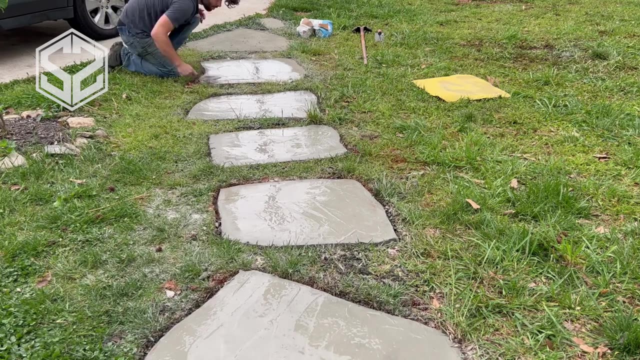 But I'm leaving some ripples in that to make it look a little bit more like a stone. When I'm done I'm going to get the paint to draw all the serious from all around the stone. I'll be adding the letters in the front directly so that when I get that little rip I don't have to make all that much of a mess. 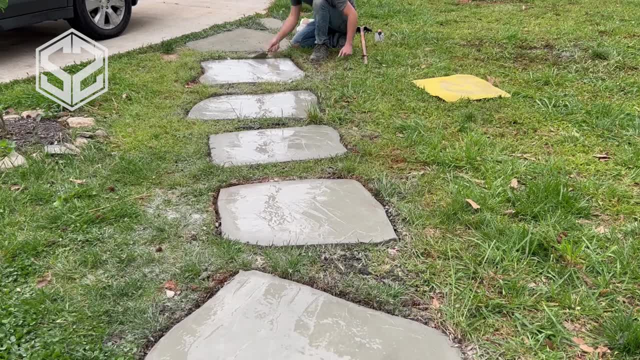 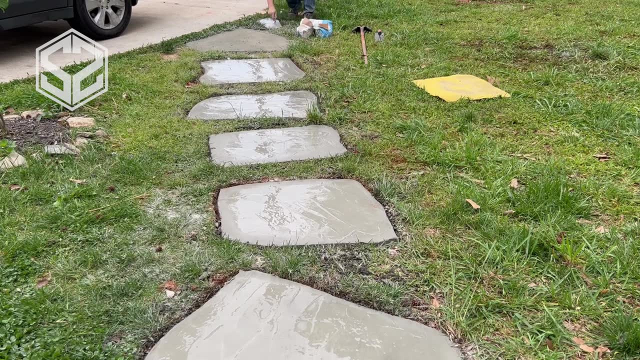 I'm going to finish it with a brownymphейr and some gold wander, But some of you might notice, after making all the trowels I only have the dots. I'll leave those characters as they are. And this For открыpiting. 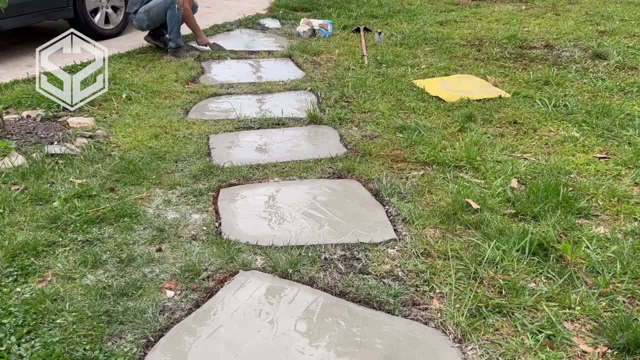 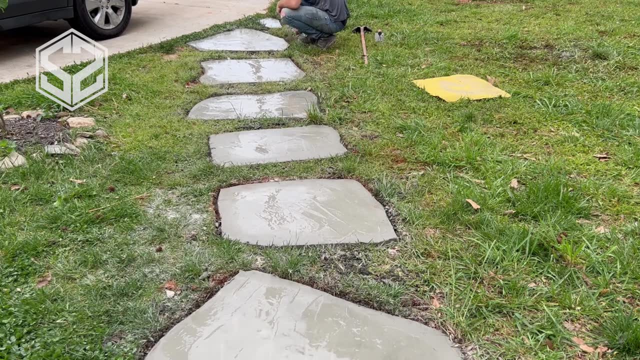 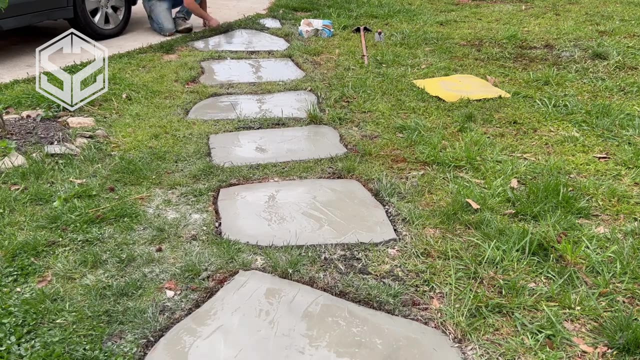 For filming, For just being students, we're very accumprove. now i've got all of the shaping pretty much done. i'm going to go through again and just add a little bit more texture to the top of each of these stones, making sure that it's about what. 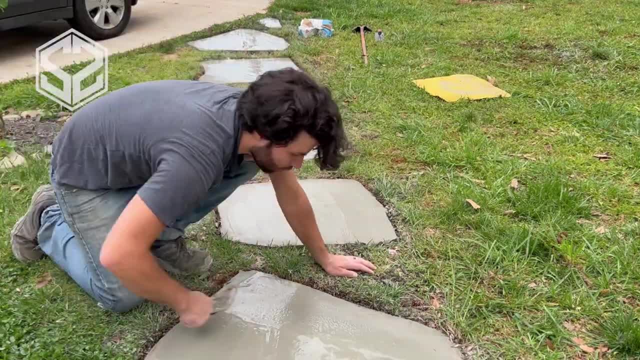 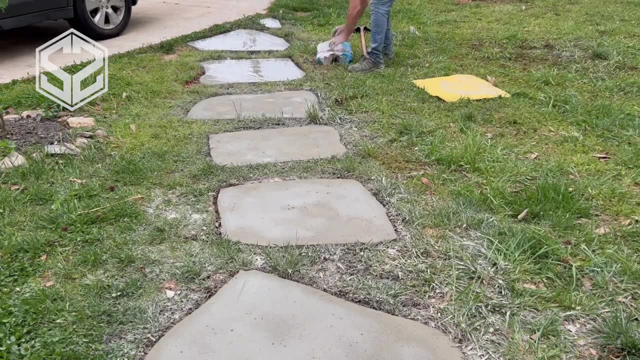 i want, and then i'm going to come back with just a very fine dusting of mortar and sprinkle that over top. my only worry about this is these are looking pretty smooth. if i don't put anything on this, it might end up being a little slippery when it rains and, as time goes by, if any moss. 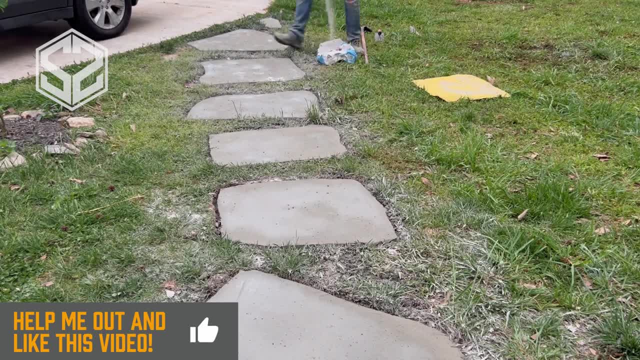 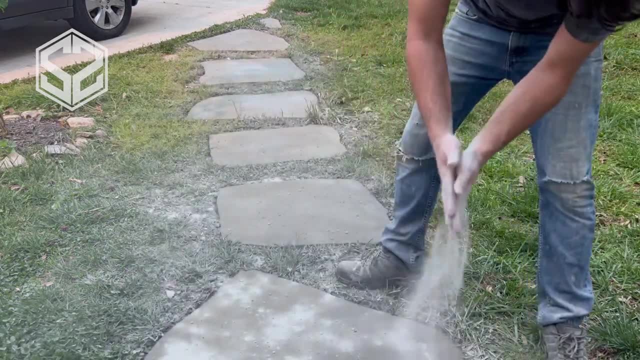 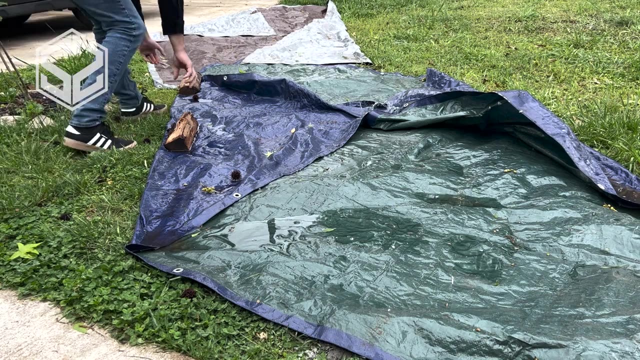 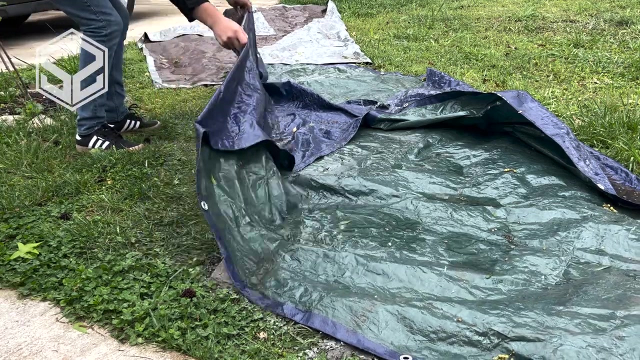 grows on these or anything. i don't want it to be too slippery, so this will just add a little bit of grit on the surface. a few hours after i finished these slabs, i had a really hard storm come through, so just to be safe i covered this up with a few tarps overnight, and now it should be good we've got a little bit more.